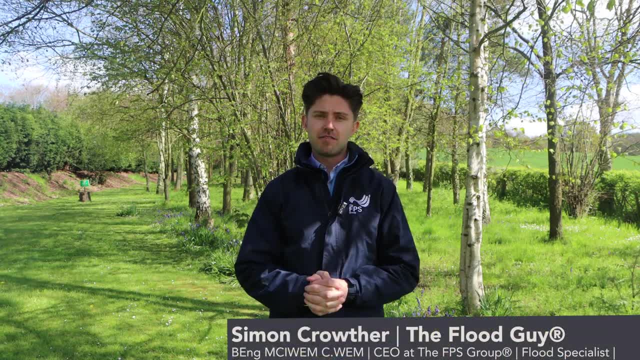 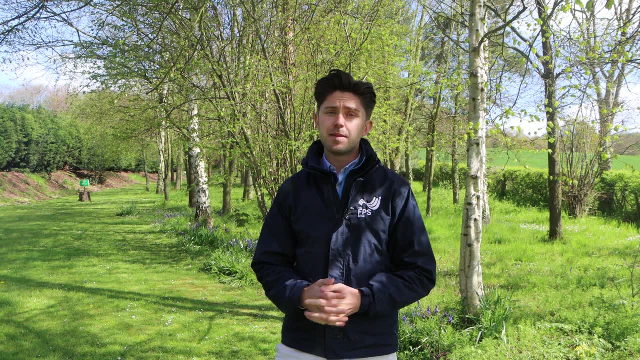 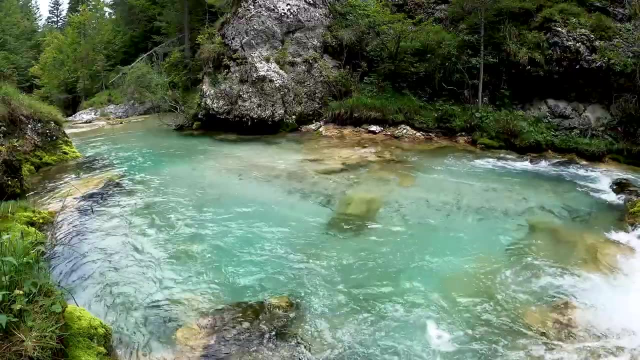 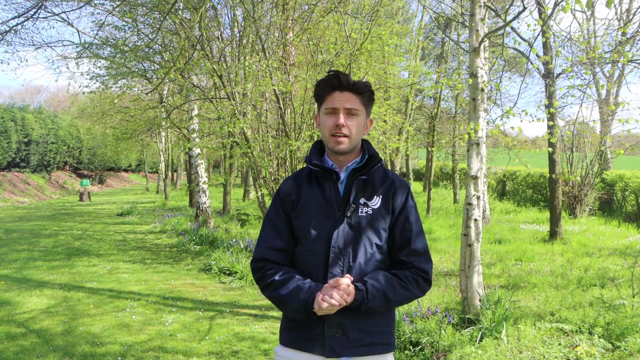 Flood modelling is the process of simulating the behaviour of flood water using data and computer models In order to forecast future flood events. flood modelling aims to predict the intricate processes that control flood events, such as precipitation, runoff, river flow and tidal patterns for different return periods, Depending on the location, risk and detail of the modelling. 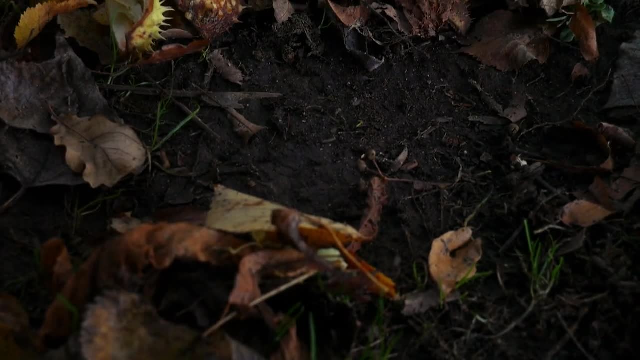 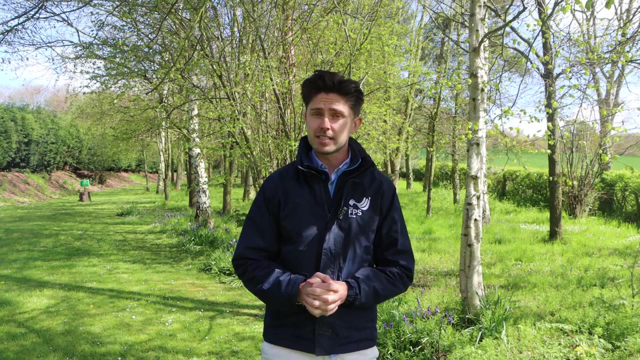 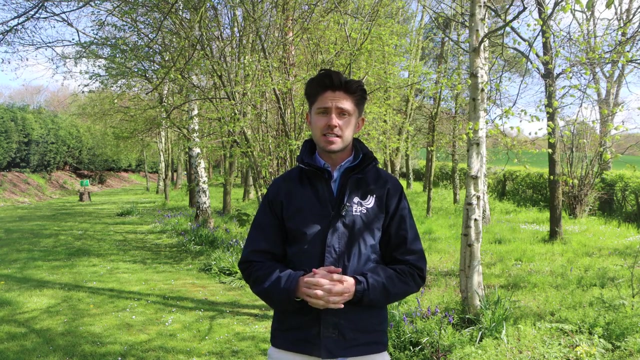 already available for your site. additional flood modelling may be required to maximise the safe development potential. If you are planning a development and require flood modelling support, FPS Environmental can help. Flood models are required when there is a need to understand and predict the potential impacts of flooding in a specific area. This could be for various reasons. 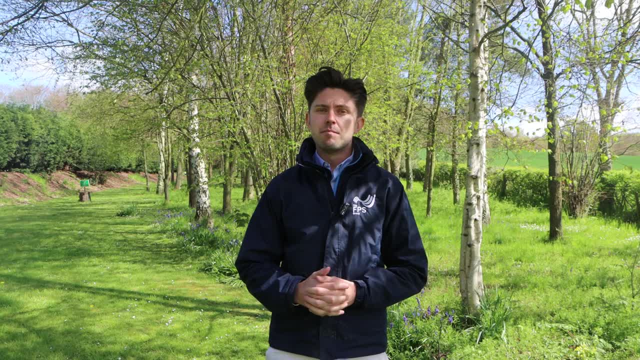 such as: firstly, planning and development Models are often required for planning applications to assess the impact of flooding on a particular area. This could be for various reasons, such as: firstly, planning and development Models are often required for planning applications to assess the 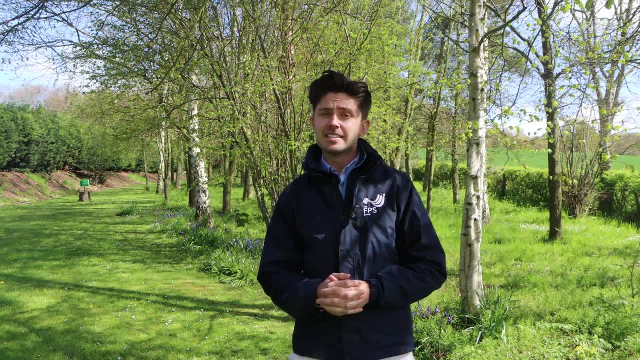 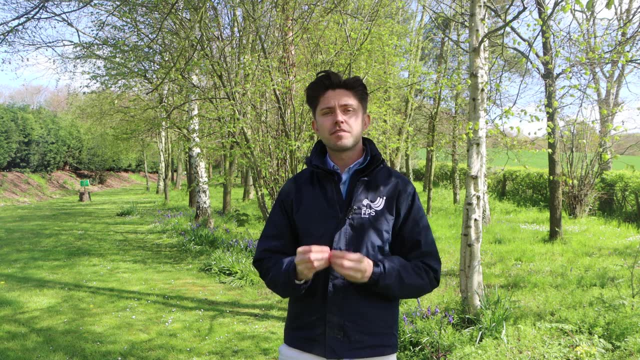 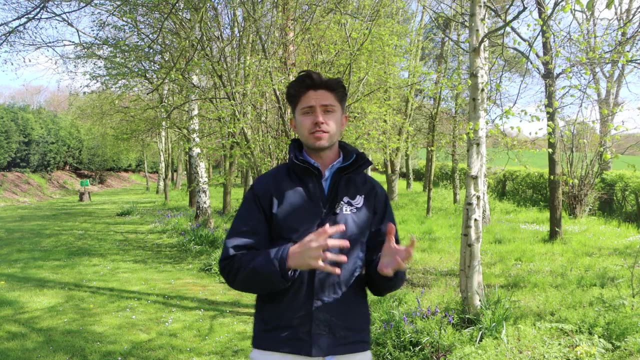 flood risk associated with proposed developments and to ensure the safety of developments and those who use them. A model may also be required to ensure that the flood risk is not exacerbated elsewhere through the development. This may include the construction of a new site or aspects such as realigning a river bank. A bespoke model may be required if existing. 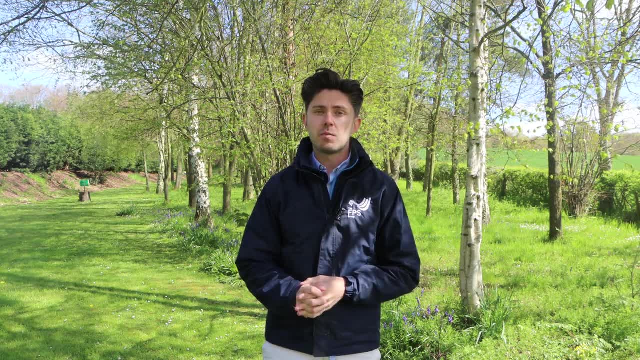 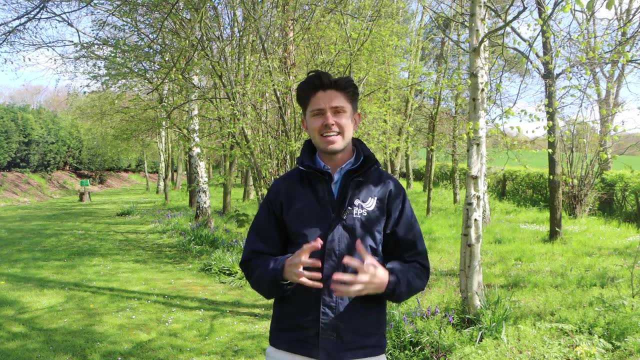 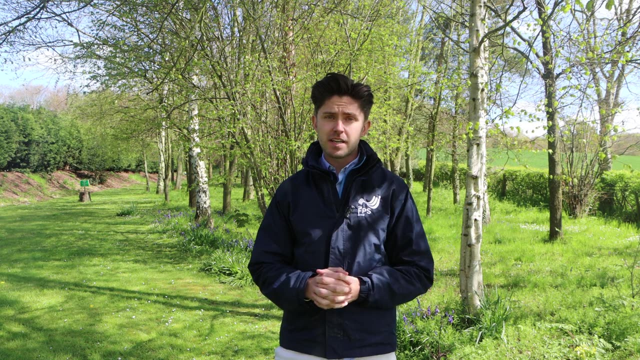 flood models are not detailed enough to make a judgement on whether or not the site can be developed safely. Secondly, another use could be for climate change stress testing and adaptation, As the climate changes flood models are used and required to understand how flood risk. 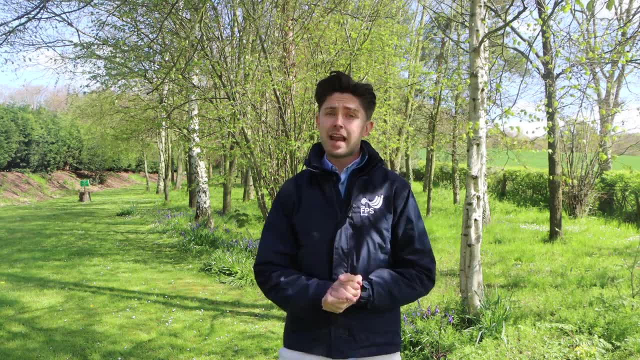 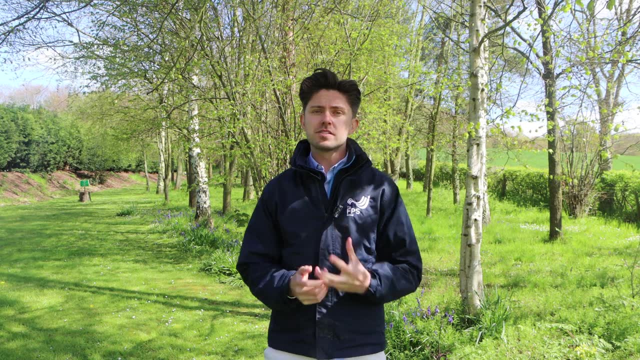 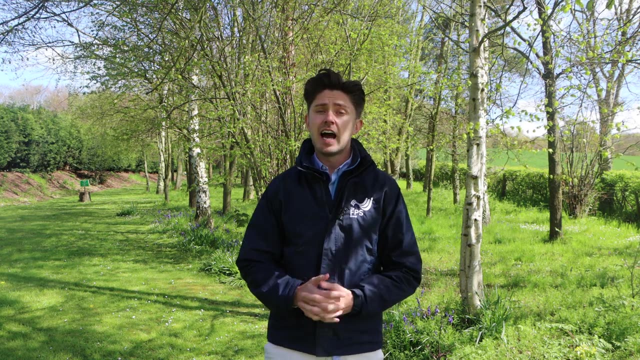 may change in the future and to inform decisions on land management practices, developments and how to adapt these changes. Thirdly, flood management Models are used to help aid decisions on floodplain management, including the identification of flood-prone areas and the development of flood maps. This information is vital not just to ensure safety. 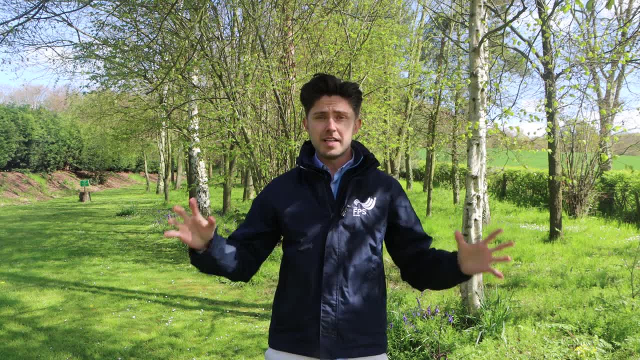 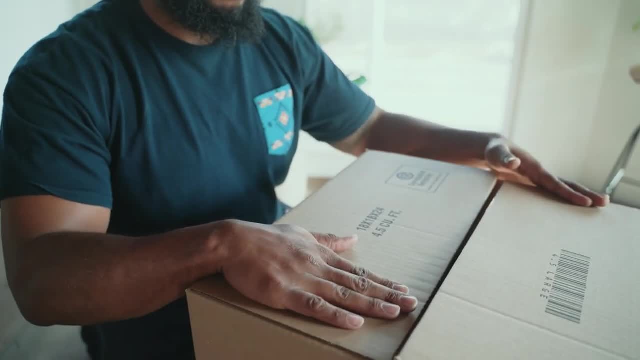 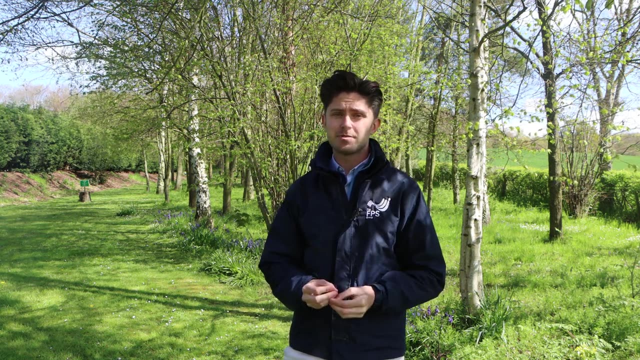 but also such that floodplain storage is maintained and that the risk isn't increased elsewhere. Fourthly, assisting emergency response plans. Detailed flood risk information is usually required to assist with floodwater evacuation plans and risk management. Overall flood models are used whenever there is a need to understand the potential risk.